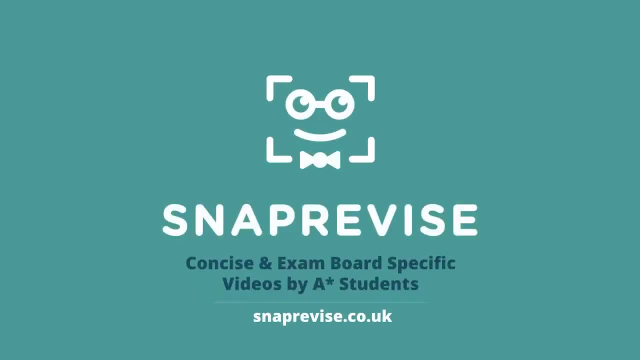 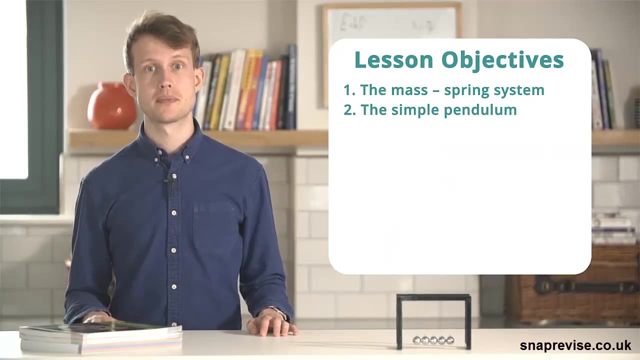 Hi guys, in this series of videos we'll start by looking at the mass-spring system, then we'll look at the simple pendulum, then we'll look at energy in simple harmonic motion and we'll finish with an exam-style question. So let's start off by looking at the mass-spring. 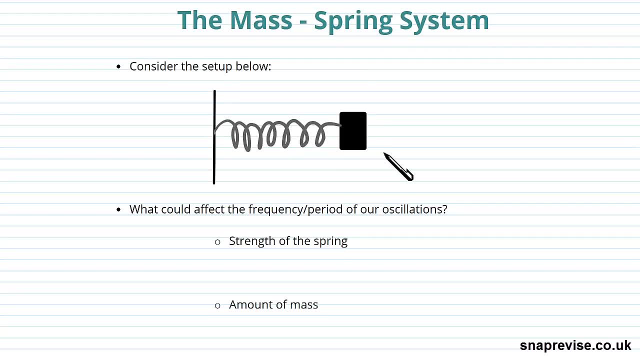 system. We're going to consider the setup below. Let's say we've got this, this spring attached. well, a mass attached to a spring, a light spring, The mass is going to have a mass of m. We're going to have the spring having a spring constant of k. We're going to say that the spring has an 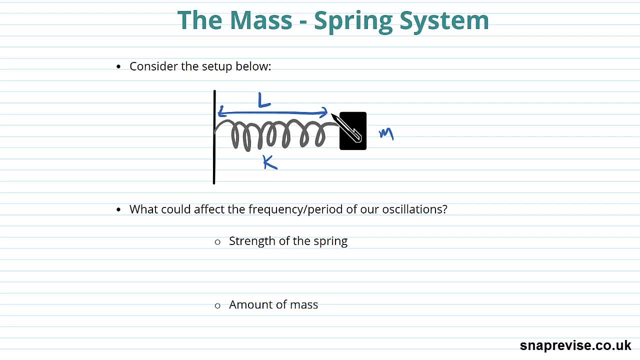 equilibrium length, an unstressed length of l, and it's going to be doing oscillations about its unstressed length, with x being the extension of the spring and a positive in this direction. Now we don't actually really need to know what the length of the spring is originally to be able to. 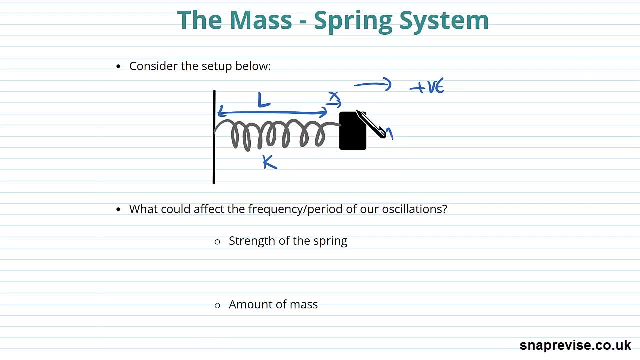 work out anything about these, these oscillations. I'm just including it for completeness, and we're going to use x to be the extension of our spring. So, immediately, what do we know? Well, we know from studying Hooke's laws previously that the mass, the block, will experience a force from the spring when we stretch it. So we know the. 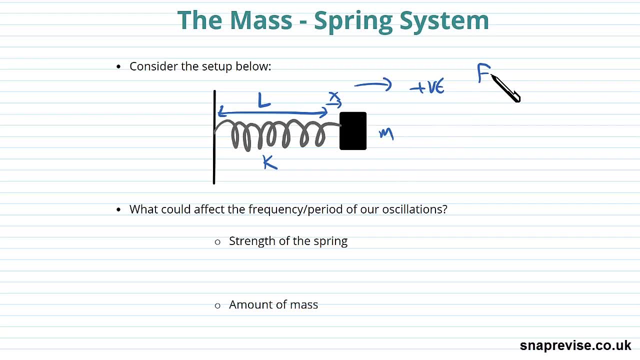 force required to stretch a spring by distance x is f equals kx, and we know that by Newton's third law. that means that the block, the mass, will experience a force of f equals minus kx on it, That is to say that the mass will be pulled back. 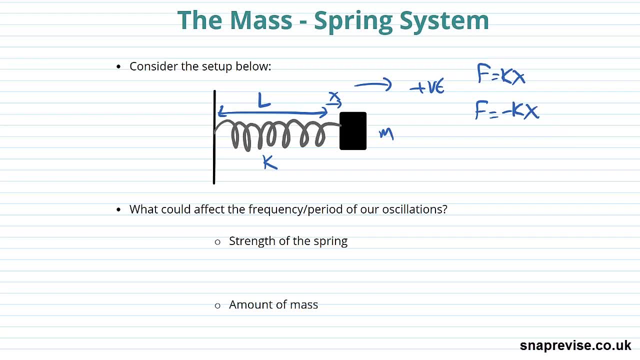 by this spring with a force of kx. So let's draw that on. So we see there's this f equals minus kx force. But immediately, what do we notice? We see that we have a force acting on our mass, where the force is proportional to the extension or the distance from the equilibrium point. 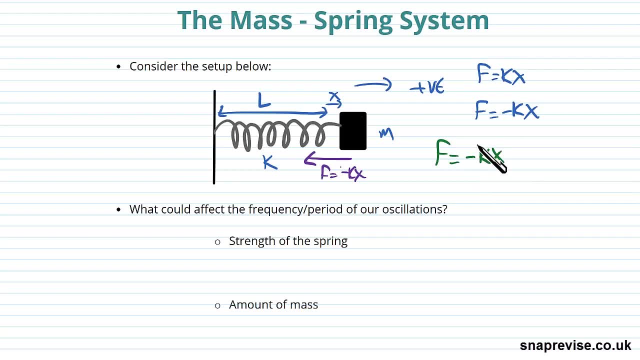 and it's negative, That is to say that it opposes the force, It's opposite to the direction, the sign of the position of the particle, that is to say, Which means we have. this is a restoring force, And so we're going to have simple, harmonic motion here, just as we talked about previously.